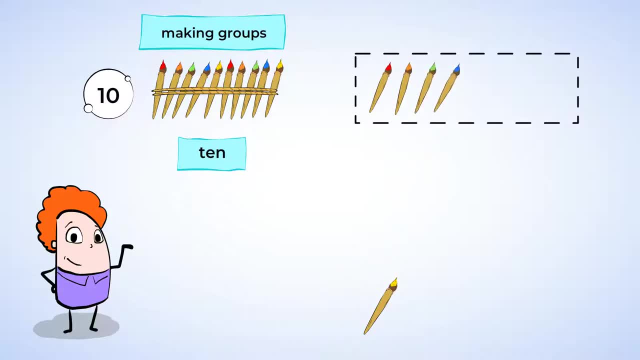 One, two, three, four, five. No, we don't have enough to make another ten. A ten must have exactly ten things in it. This group of ten is called ones. so we have one ten and five ones. but we were counting. 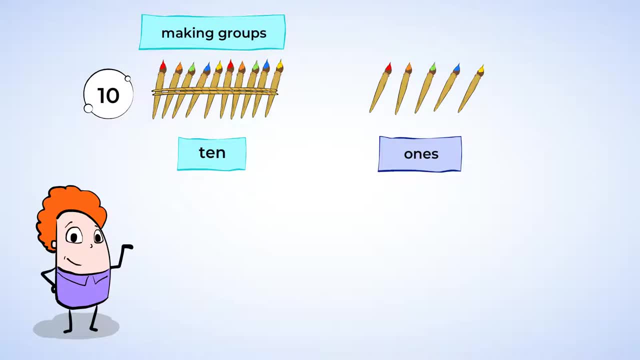 here, right? What number is that? Let's look at this special chart that tells us the number. This side says tens and this side says ones. Under the word tens we write how many groups of tens we have. We have one group of ten, so let's write the number one. 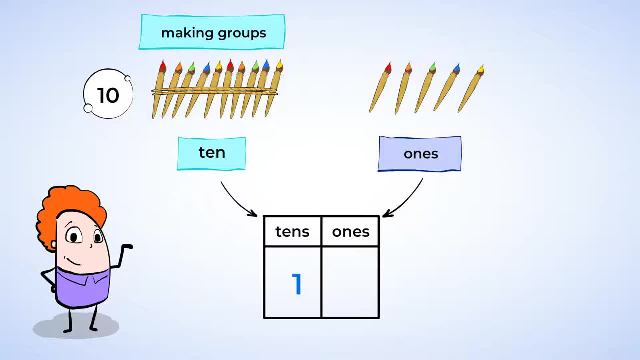 One, two, three, four, five. Under the word ones we're going to write the number of single paintbrushes we have. We have five paintbrushes, so let's write that number here: five. Can you read the number in the chart? 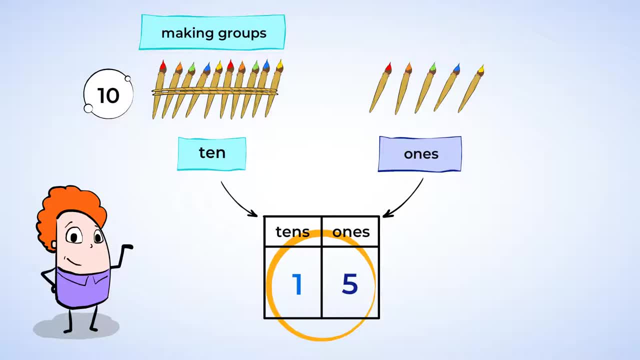 It's fifteen. This means that one ten and five ones is actually the number fifteen. Just to be sure we can check this by counting. We already counted the group of ten, so we don't need to count that again. We can count on from there. 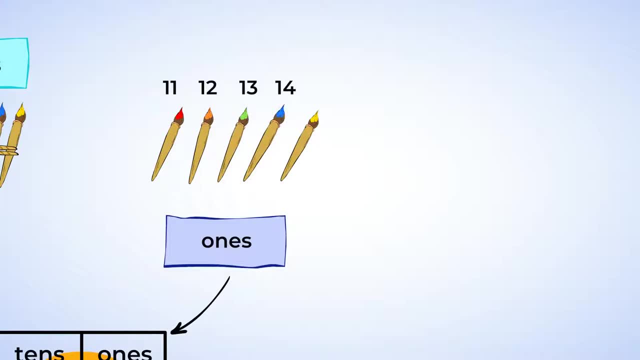 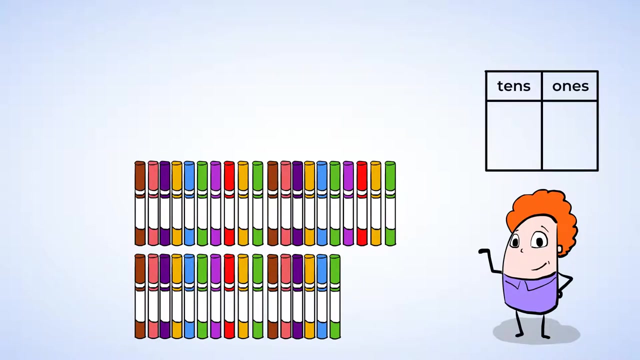 Eleven, twelve, thirteen, fourteen, fifteen. We have fifteen paintbrushes. Now it's time to move on to the markers. Just like before, we're going to make groups of ten. to help us count quicker, Let's start by counting one group of ten. 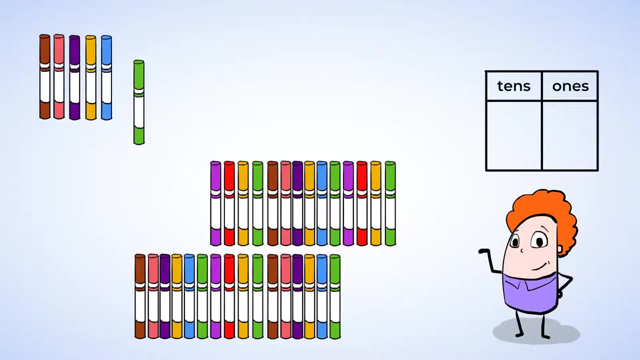 One, two, three, four, five, six, seven, eight, nine, ten. That's one group of ten. It looks like we have enough markers to make more groups of ten. Let's start by counting one group of ten. 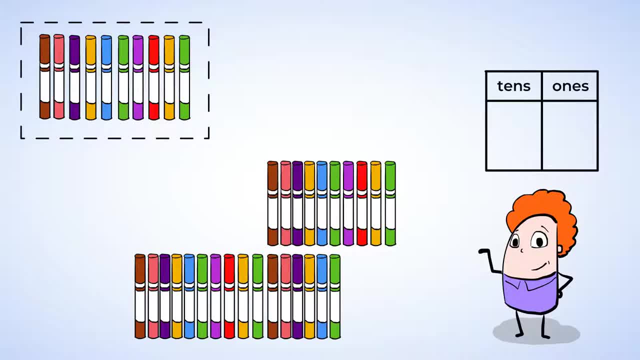 One, two, three, four, five, six, seven, eight, nine, ten. That's one group of ten. What do you think Let's try? Here's another group of ten And another group of ten. How many groups of ten do we have now? 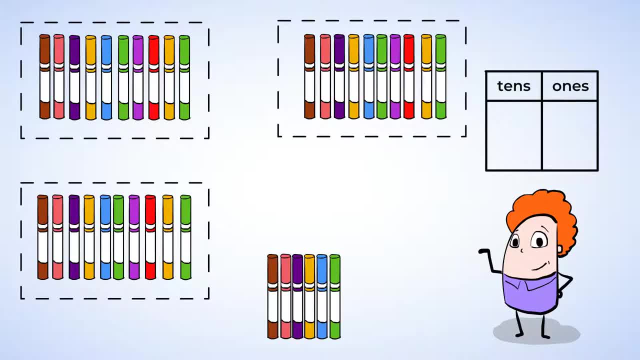 Three Or three tens. Write the number three in the chart in the tens place, And how many ones are there: One, two, three, four, five, six. There are six ones. Write the number six in the ones place of the chart. 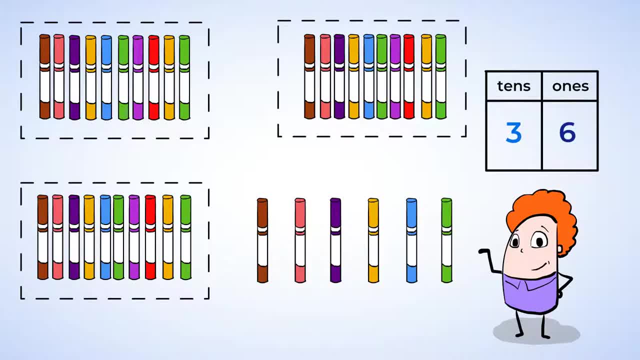 And can you read the number in the chart? It says: That's right, Thirty-six. This means that three tens and six ones is actually the number thirty-six. But just to be sure, we can check this by counting First. count the tens. 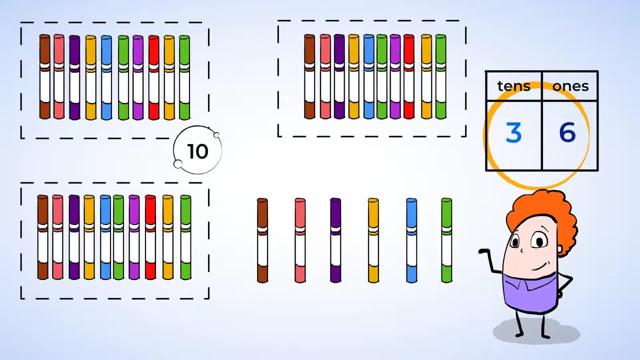 Because each group has ten markers, we should count by tens. Ten, twenty, thirty, And now we count by ones. Thirty-one, thirty-two, thirty-three, thirty-four, thirty-five and thirty-six, And now we count by ones. 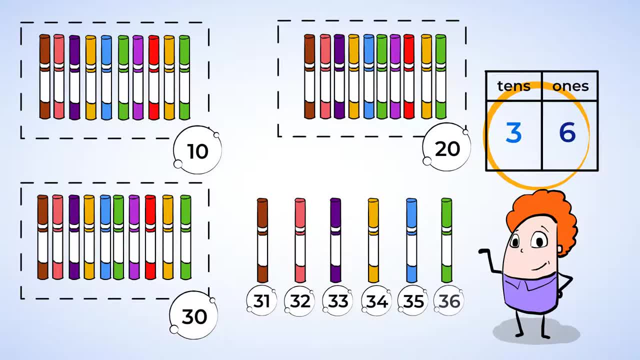 Thirty-one, thirty-two, thirty-three, thirty-four, thirty-five and thirty-six. It says that's right, Thirty-six, 36.. You have 36 markers. You're doing a great job counting tens and ones. And now, last but not, 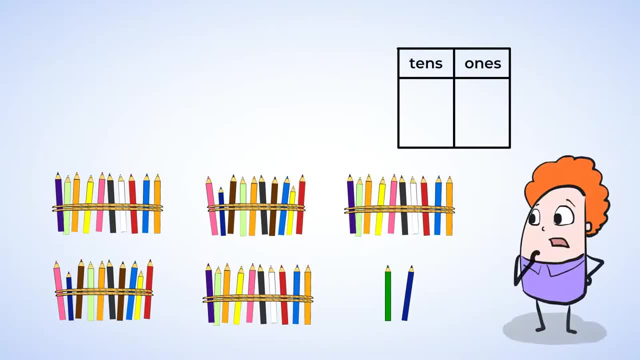 least. let's count the colored pencils. Wow, there are a lot. How many groups of 10 are there? One, two, three, four, five? There are five groups of 10, or five tens. So we're going to. 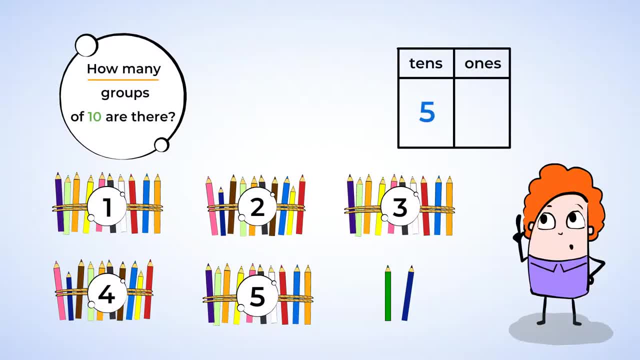 write the number five in the chart under the word tens. And how many ones are there? One, two. There are two ones. So we write the number two in the chart under the word ones, And what is the number in the chart? Fifty-two. But let's check. 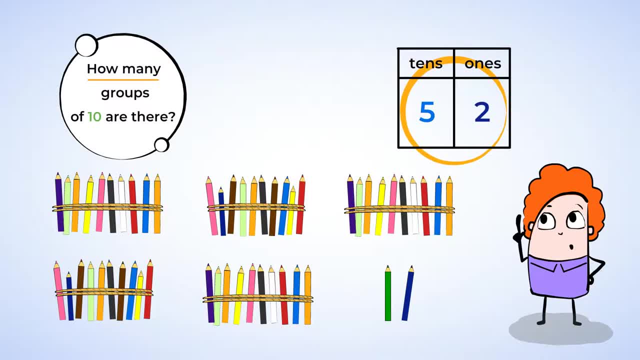 First we count the tens. Because each group has 10 colored pencils, we should count by tens: 10,, 20,, 30,, 40,, 50. Now we count by ones: 51,, 52. Yeah, you have 52 colored pencils. 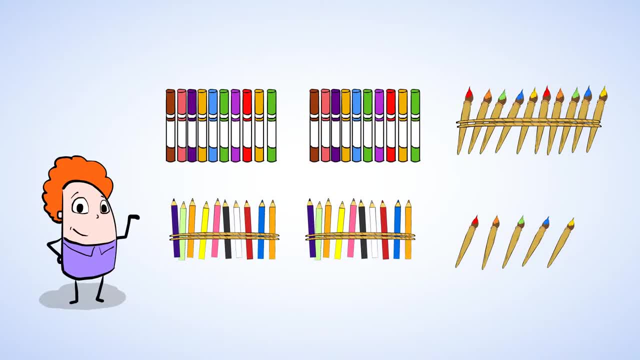 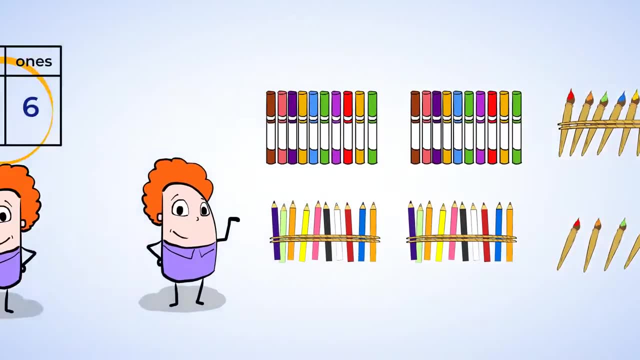 We just counted up all the art supplies so quickly. I can hardly believe it. Way to go. Now they're organized and ready to go. Now they're organized and ready to be used for fun art projects. We've just learned that counting is easier by making groups of 10, which are called tens. 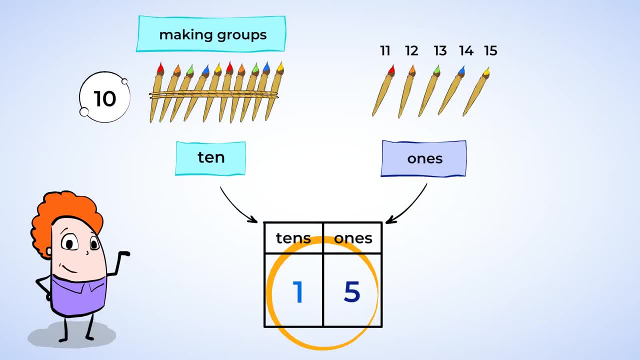 If you don't have enough to make a group of 10, those are called ones. We can write the number of tens and ones in a chart and then read the number to know how many objects we have. This is a very important skill, so we'll keep practicing it together.